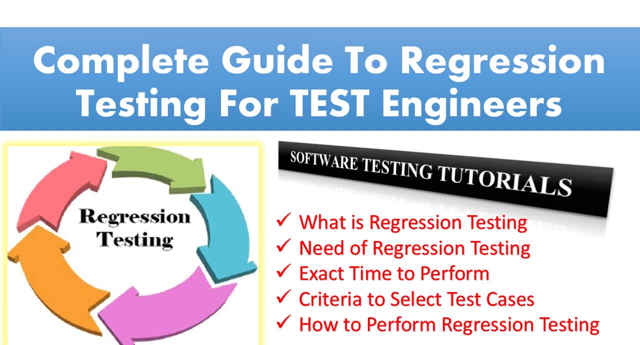 perform regression testing. so in this complete guide to regular testing, so i'm giving a complete regression testing concept with the help of examples, and so in upcoming videos you will learn how to prepare the regression testing test cases and how to select the major test cases, which is impacting our application. so let's get into this concept. so let's start. what is the regression? 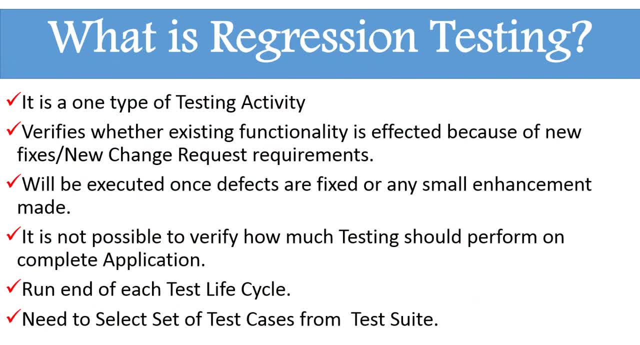 testing. so everyone know that it is a which is a type of the testing activities we are performing day-to-day life. so which is a testing activity means we are performing the testing on a web applications or mobile applications or any desktop applications. so which is a one type of testing. 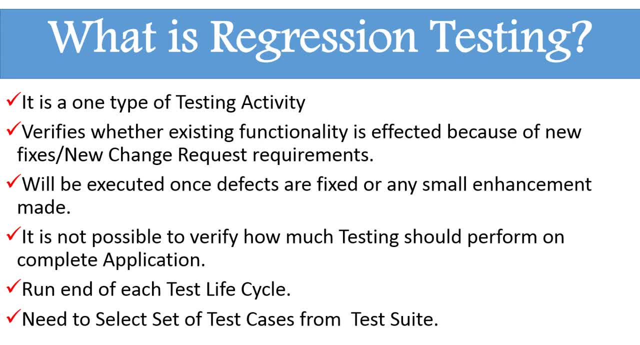 functionality activities. so what it will do? it will verify whether existing functionality is affected because of new fixes. so what are the functionality? we are already tested and reported the defects. because of those fixing the defects, any new defect is raised and we are getting defects in different modules, like we are having four or five models. customer registration. 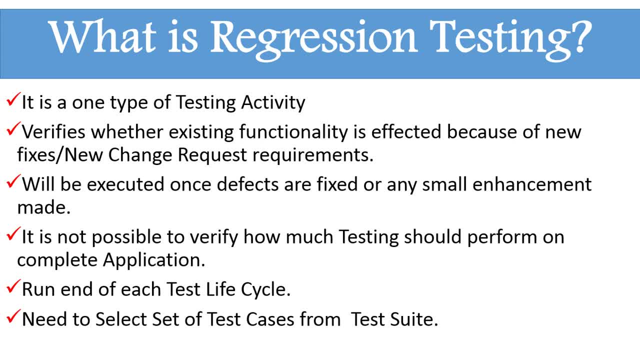 customer update and creating the new cards and checking the customer details. so suppose you have raised defects in manage customer, like creating the customers. so defects has been fixed. but very you verify the complete functionality in update customer, you will get some error, like you are facing some issues in update customer so you are not able to update. so this is called. 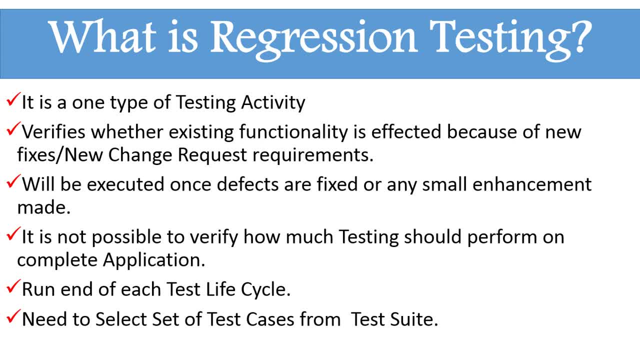 the retesting. but whenever you are performing the testing of additional functionalities then it will call as a regression testing. so we will get deep into those. and next point is new change request requirements. whether in between any new change cr request comes and developer has introduced those requirement in current build release. so then you have. 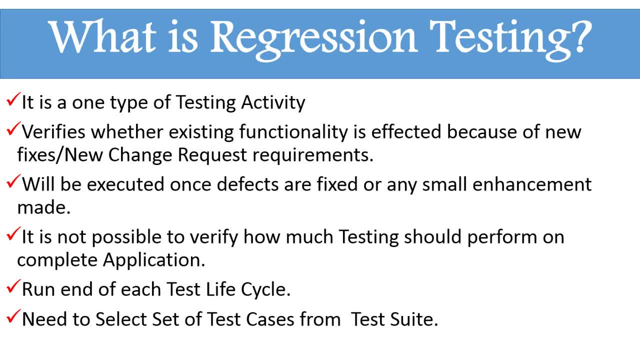 to test each and everything. so regression testing will be executed once defects are fixed or any small enhancement made. so, as discussed in second point, suppose, when you have to made execute, the regression testing means, so defects are fixed, everything is done, and at the time you are performing retesting on those defects, so defects are. 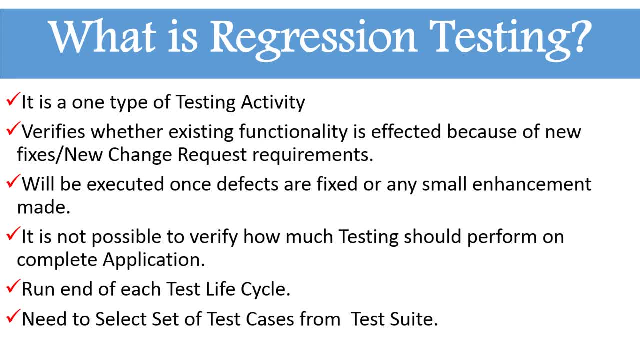 closed and some defects will be reopened. so then after that, as well as retesting those defects, you will perform on complete application, right. so our second one is any small enhancement made. so because of new change request. here we are adding developers, adding any enhancement, like adding the fields and adding the buttons, and adding those, some success messages and 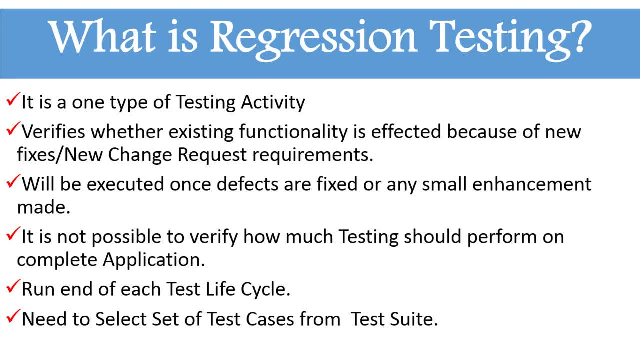 redirections. so because of this, you will get effect. so and regression testing is not possible to verify how much testing should performance on complete application. so why we are regression testing is doing means we have no idea like how much testing we have to perform. so why? because any tester can't say that your application 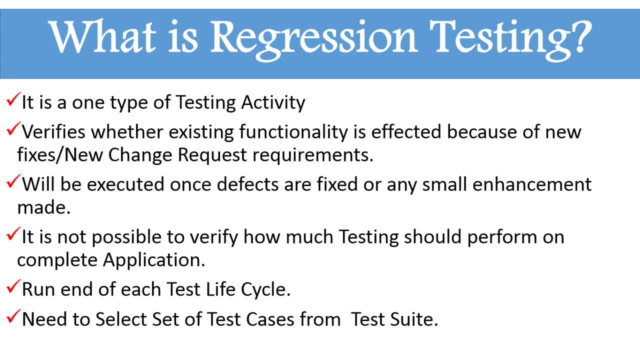 is without bug free application. it is a not a bug free application. this is not possible. why? because So when we are testing, we are testing only single bugs. So we get bug free application. because because we have no bug free application and these users and two, three, five, a maximum 10 users- but in production multiple users- are using. 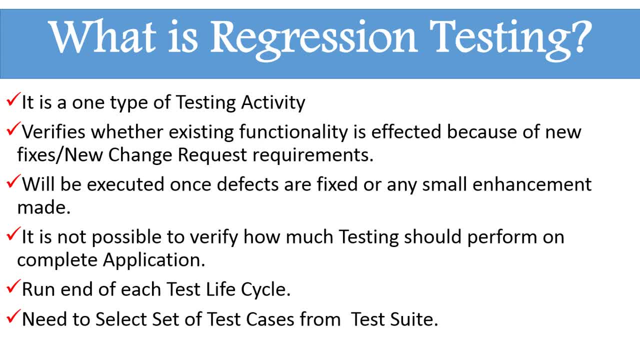 those applications. So at that time, what happens when you are consuming the rest API web services or any services from any integrated applications? at that time you will get slowness. So because of slowness, the response will take so much time. 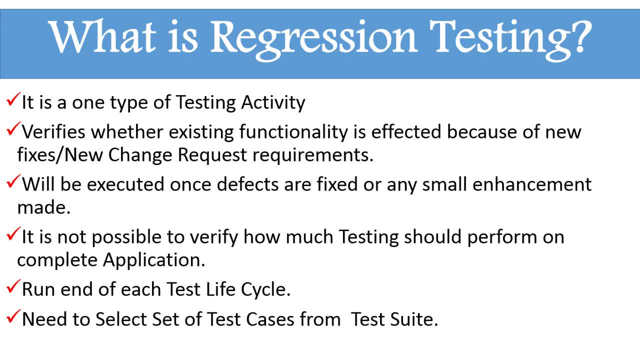 We are performing performance testing. that is different. but coming to manual testing and functional testing and the applications it will, you can't see that you will not get any defect. So that's why it is not possible to verify how much testing should perform. 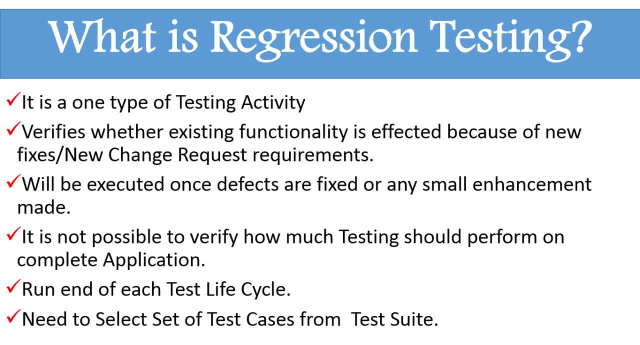 So regression testing will be run end of each test lifecycle. This is called as a normal regression testing. We are having two types of regression testing. One is a normal regression testing and final regression testing. Okay, What are the regression tests I'm running after each test? 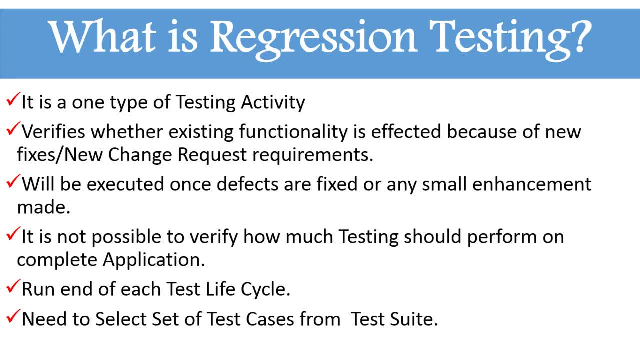 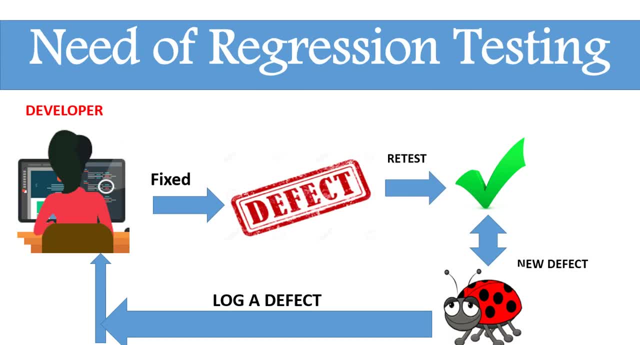 I guess this is a normal regression flow. Okay, So need to select the set of test cases from tests. So why, when coming to regression testing, we need to select the set of test cases which is high priority test cases. Okay, 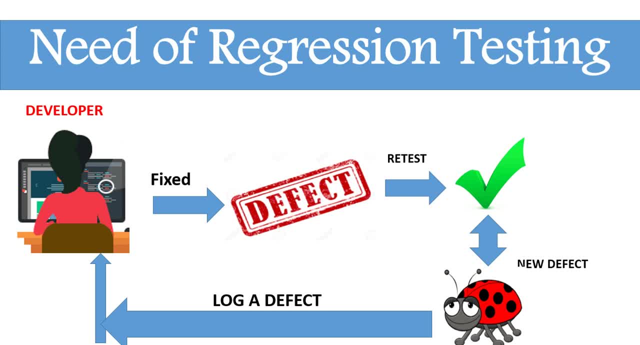 From the test suit. So why we need to verify those test cases only in the form of regression testing? This one we will discuss in next lesson. So why? Because if you don't know how to select the test suit, Okay, If you don't know how to select the test cases for regression testing, you can't perform. 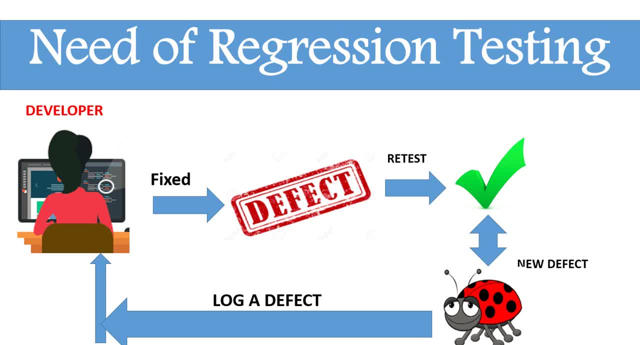 any regression testing and you can't say that this is done for regression testing and this is done for manual functional testing. So that is very important. So, moving on to next, So what, what is the need of regression testing? So let me have given one diagram. 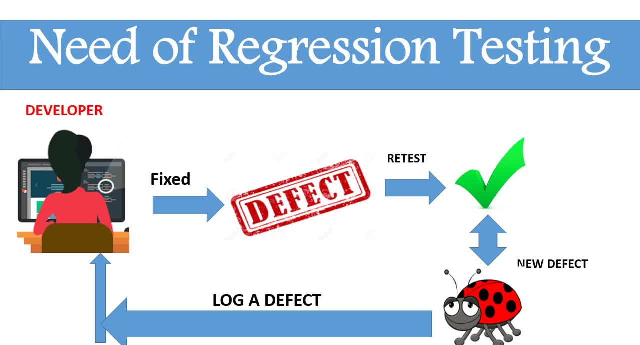 You can see here: see developer fix the defect. see developer has fixed the defects. Okay, What are the defects We have raised on some tools like test management tools? He has fixed and he has email. So once defects is fixed, he has given the build release note. 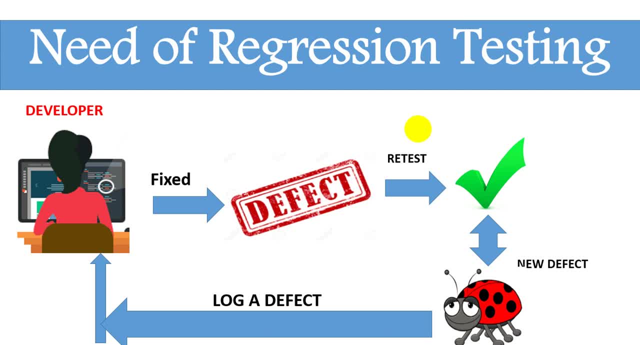 These many defects are closed and we have retested those defect, right, Sorry, We have retested those defect and we are saying that that is working fine, which is closed, So it is not reopen, which is not uh like, uh, reopen and defer something duplicate. 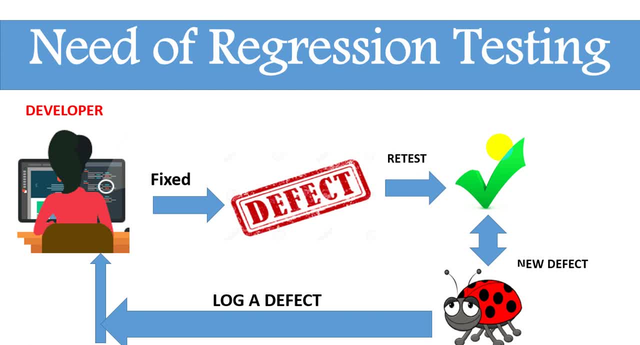 So that is working fine. But what happens? We are not saying like once defects are fixed and we have retested, means application is working properly. Not, we can't say that. So why? Because we have to test another model. also, What are the dependency modules? 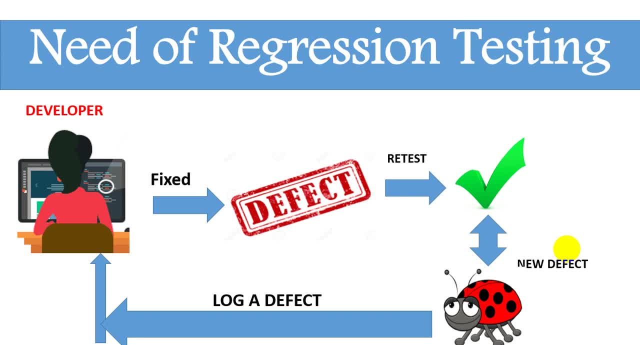 Just like I have given an example, right, Okay, Customer can create, Customer can update, Customer can change those mobile numbers, Customer can uh and uh delete and he can and uh, you can cancel those accounts. 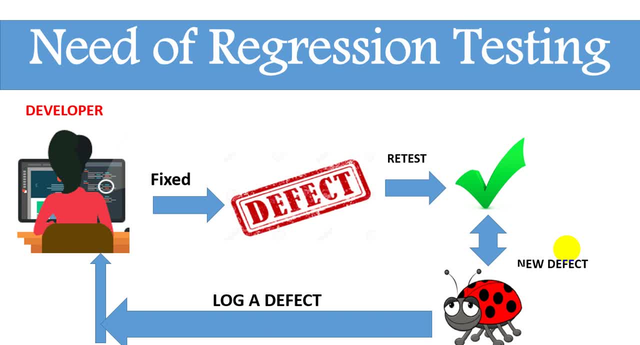 So these many, we are concentrating on those means. that is a major functionality. If because of these changes, retest defects, any defect is introduced, So because of that any introduces defect introduced, that is a new defect we have given effect. 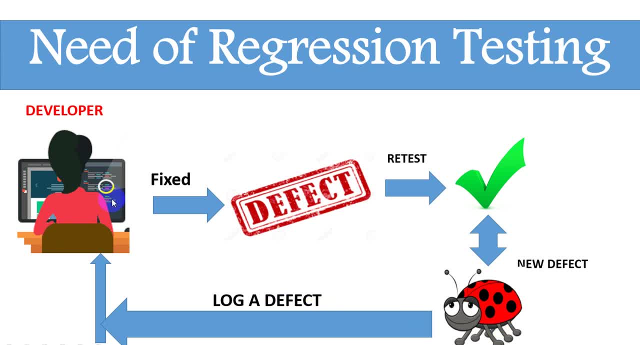 And again lock the defects, But then It is going to develop it. So these cycle will be happening every time. So because of this cycle, what happens? You can't a hundred personally say that this application functionalities defect, free application. You can't say that. 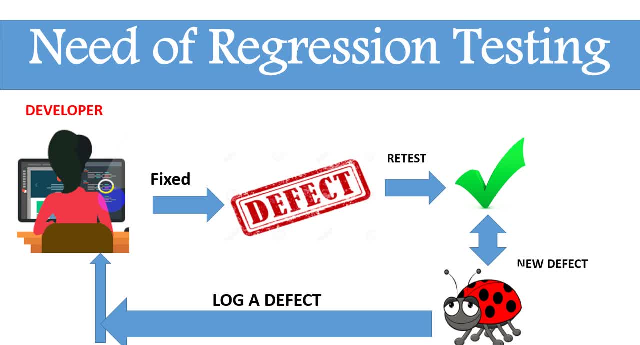 Why? Because when you perform regression testing, then only you can say that this application will be defects. free applications. Why? Because regression testing, having separate test cases, which is very high priority, and most of the times we have to perform those regression. 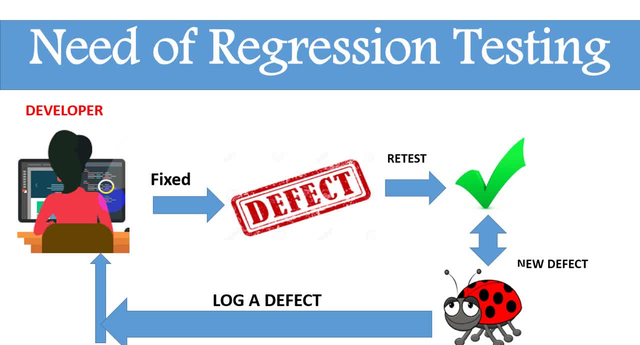 So those test cases where is repeated actions will be happening on the applications. So I will give you one simple flow: manage, cause greater customer, update customer and you can perform. select the product and you can perform payment gateway Those payment you are doing. 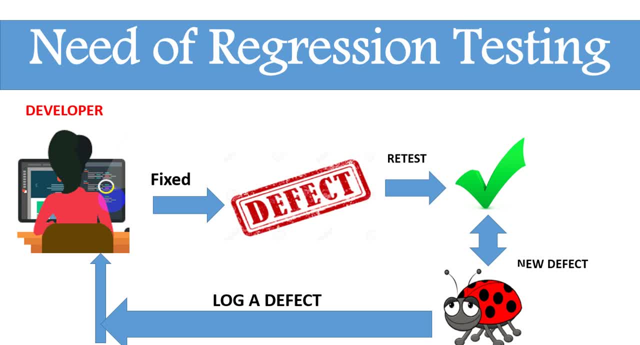 So when are the diff? we are facing defects in customers and product selections, right. So when coming to customers and product selections, Right. So when coming to regression testing, we have to perform entire flow. So why? Because if customer has changed those details whenever he is doing the payment in that payment. 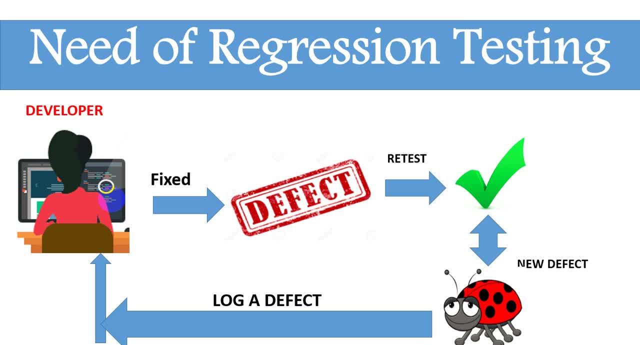 receipt. we are seeing those customer details updated details. If it is updated it is not there, The customer will not receive any product which has he which he has purchased. So there we are getting one defects right. That is a regression testing. 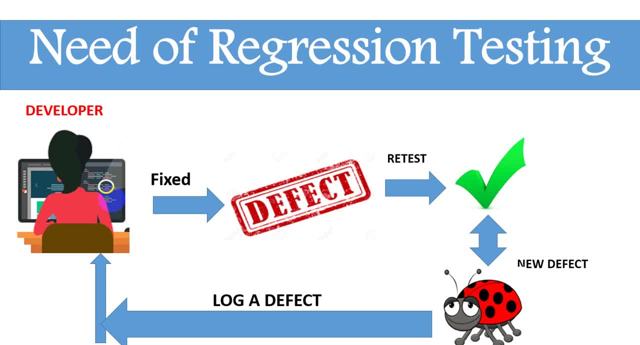 You have to perform complete flow that dependency: manage customer, update customer product selections and add to cart. These are all are integrated and dependent, which is dependence for payment gateway. Because of this payment gateway, we have to perform these all many cycles compulsory.